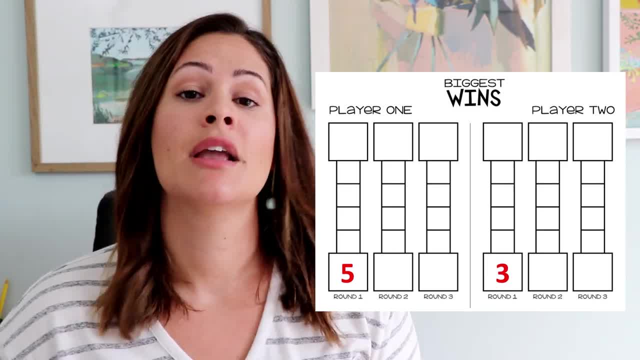 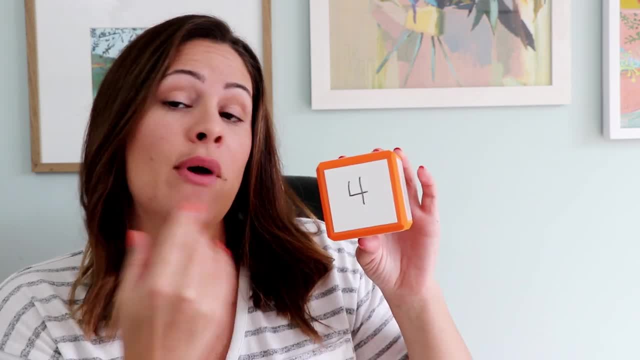 ahead and roll their dice Three. As students continue to go ahead and roll that die, they're adding on to the number they had before. So player one just went again. they now have a four, but they're not going to write four in the box above. They're going to 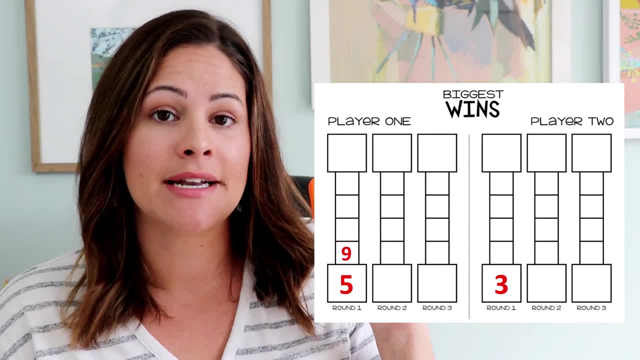 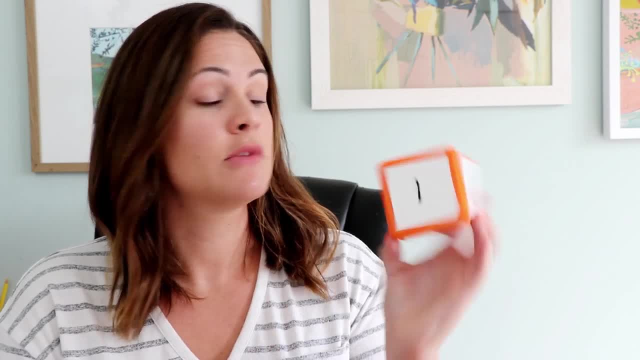 add the four to their five and now they have nine. Their new sum is nine. They will write that down in the next box and pass the die. Student two will go one. One plus three equals four. They will write a four there. Students keep rolling and adding back and forth until 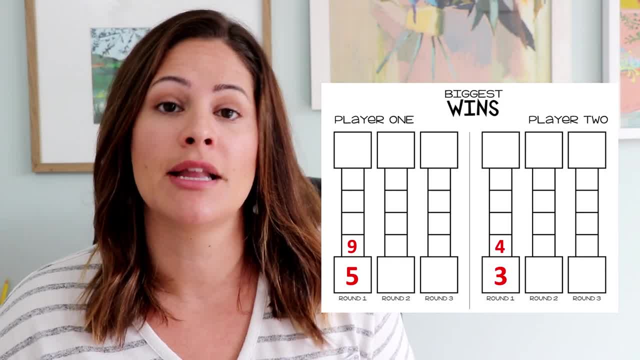 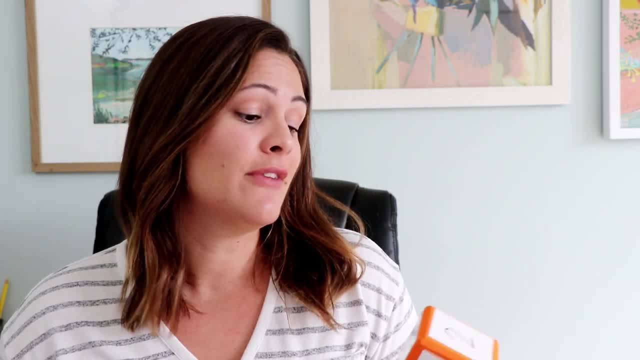 they get to that top box at the end and whoever has the biggest number in that box wins, Hence why it's called biggest wins. This game is really great for first grade students To play, because if you rolled six, all five times, the highest number you could get is 30. So most of 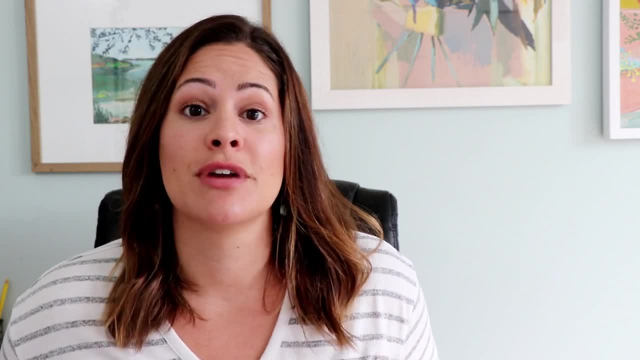 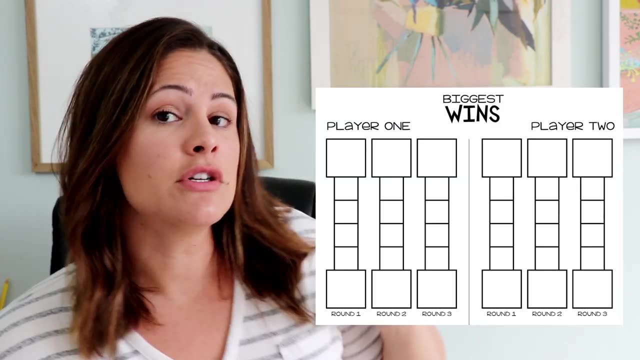 your addition is going to be between one and 30, which is great for students to practice. To make this game a little more difficult. it's actually pretty easy to ramp up. So here are some ways you can do that. First, there's the box at the bottom here, and that box you could actually, instead of 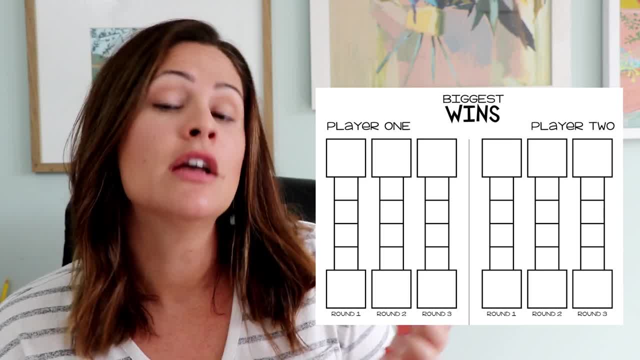 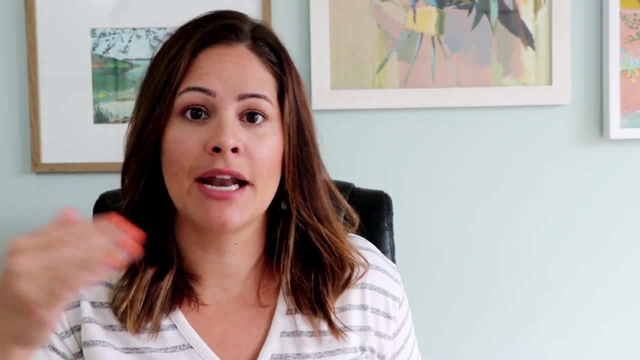 leaving it blank and waiting for the students to roll. what number will go in there? you can go ahead and choose a number to start with, So you could have it start at 40 or 50 or 20.. So then, students are adding on higher numbers. You could also have students use two dice and they 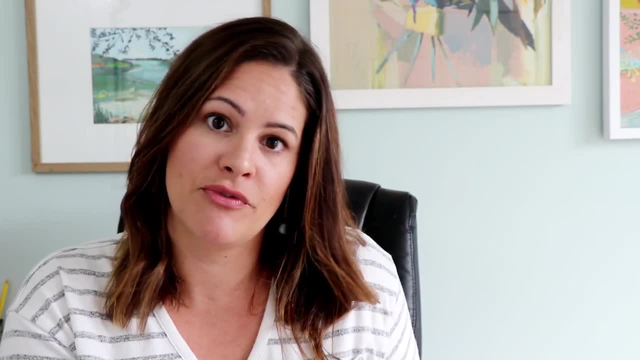 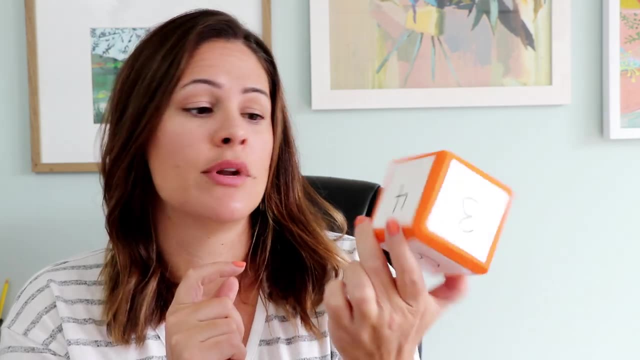 need to find the sum of the two dice and then add it to the number before. That would ramp up those numbers pretty quickly. Or you could easily take a dice like this- These are the dry erase ones I've shown in the past- and you could go ahead and add all different numbers on here. It doesn't need to. 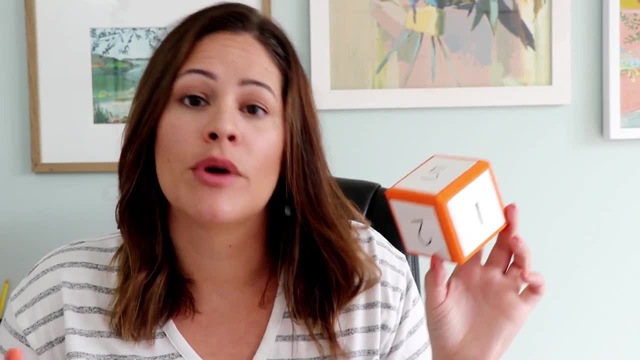 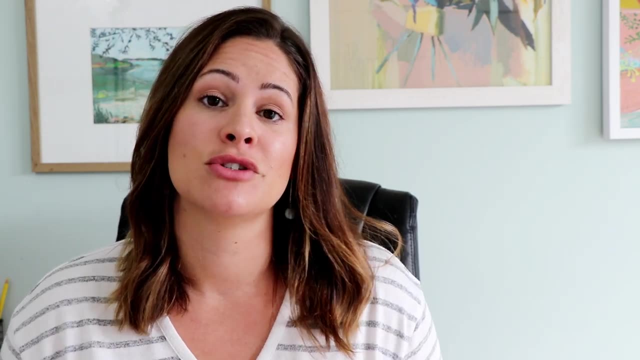 be one through six, So you can have seven, you could have ten, whatever you want. Doing this can help differentiate this game for different levels of learners in your classroom, or for just you and grade teachers, who find that one through six might be a little too simple for them. So that's. 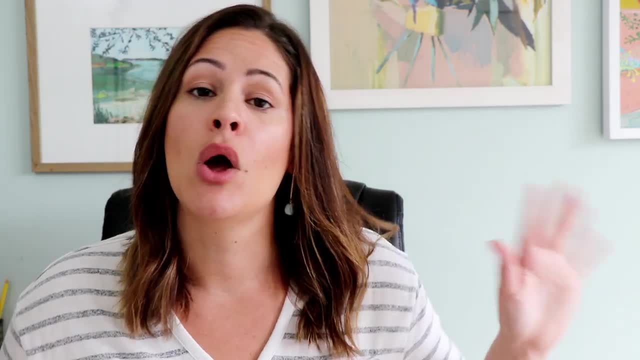 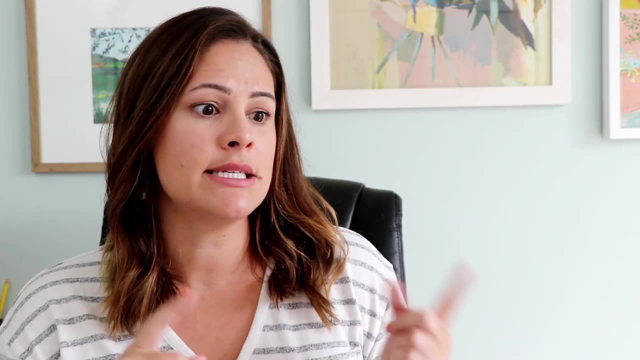 the game Biggest Wins and players can do the best of three rounds to see who wins the prize in the end. That game is simple enough, but I want to show you that I actually have another version. So the Biggest Wins is included in my addition print and play unit because you're practicing addition. but